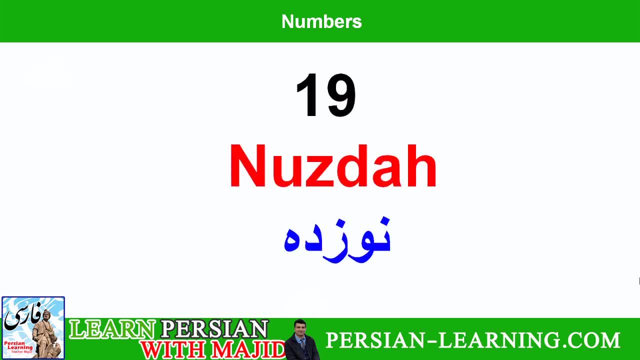 Nineteen, Nineteen, Twenty, Twenty-one, Twenty-one. From now on you have only O here, which means and which means twenty and one or twenty-one. So you can continue with twenty-two, Twenty-two, Twenty-two, Twenty-two, Twenty-two, And so on. 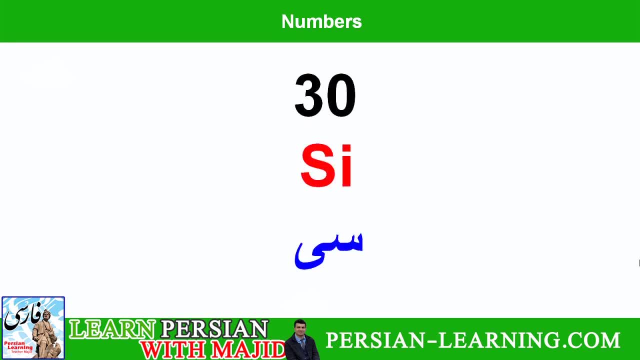 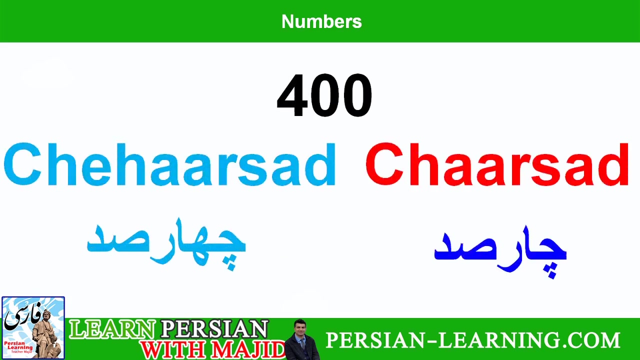 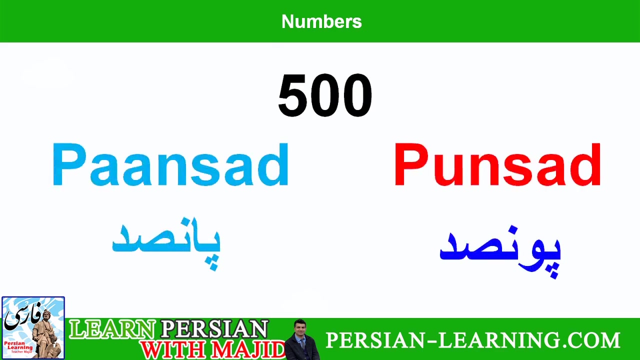 Thirty, Thirty, And also you can say thirty-one, Thirty-one, Thirty-one, Forty, Fifty, Sixty, Seventy, Seventy, Eighty, Ninety sat sat, divist, divist or divist, which is the formal version: chahar sat, chahar sat or chahar sat, pun sat, pun sat or pan sat, shish sat, shish sat or shesh sat. 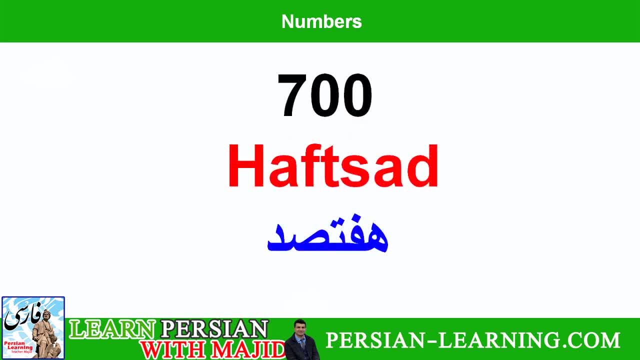 haf sat, haf sat haish sat, haish sat noh sat, noh sat hezar, hezar, do hezar, do hezar, and then you can continue with se hezar, chahar, hezar, panj hezar, and so on, milion, milion, yek milion. then you can have: 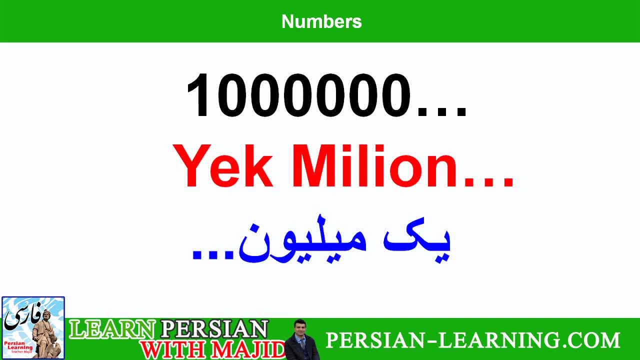 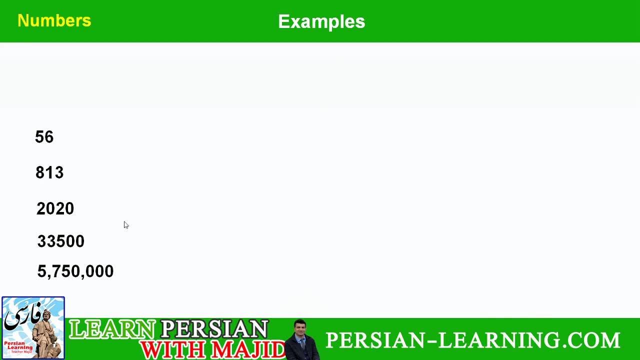 milion, do milion, se milion, and so on. let's have some examples how to read these numbers in persian. so we have 56, what is 50? it is panjah. then you have six in between you must have, and which is all in persian. so we say: panjahu shish. here we have 813.